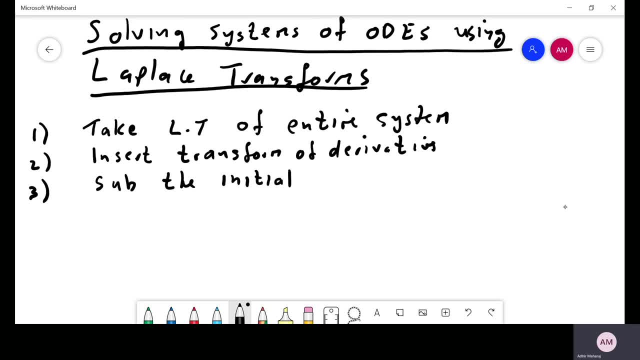 Substitute the initial conditions and simplify The fourth step. now, when you're dealing with a system of- Okay, differential equations, obviously you'll have more than one dependent variable and since they are od is, you'll only have one independent variable. so to solve for a specific variable at a time. 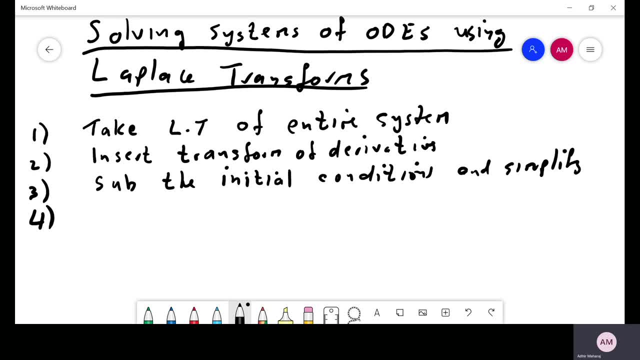 there are many ways you can do it, like simultaneous equations- right, is one of the ways, but i refrain from using simultaneous equations because it takes too long. what we would use is kramer's rule, right? so then we use kramer's rule to solve for the variable. 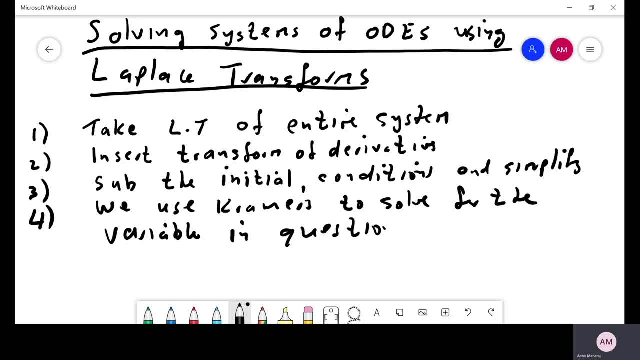 in question and once we do that, use inverse laplace transform, inverse laplace transform to obtain the solution. the solution, okay. so if you notice the steps, is similar to solving single equations. however, there's one extra step there where we're going to use kramer's rule. right for this course, you'll 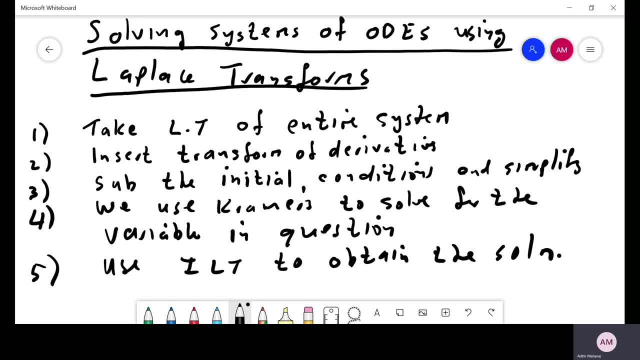 only work with systems of two equations, for me. we won't go to three equations, we'll just go to two equations. uh, because the method is the same, it just takes longer to do so. we will follow this method with the following example that i'm going to put up: 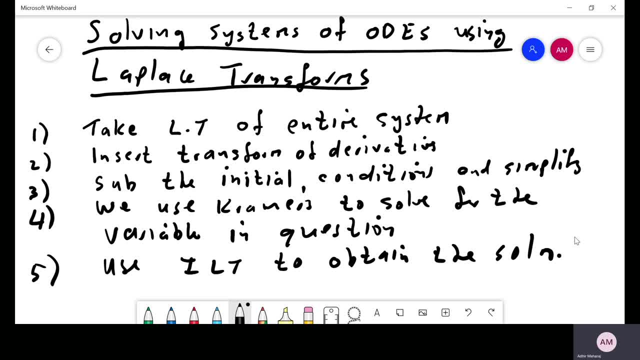 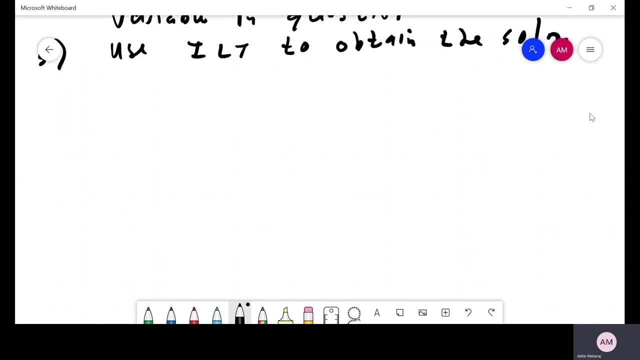 and uh to show you how to find the laplace transform. using laplace transform to solve systems of equations. so let's put an example up. so, example one. well, i'm just doing one example. so they create the system of equations i'm dealing with is x, dot. 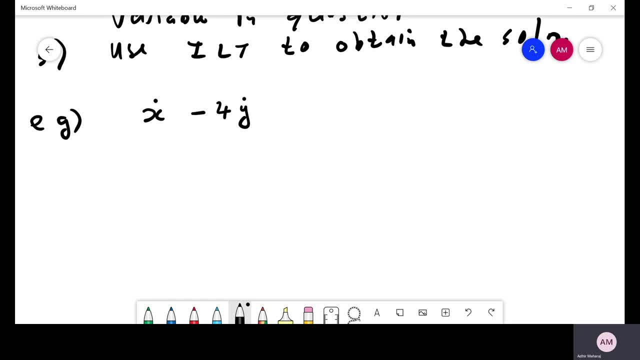 minus four y dot. the dot is derivative with respect to the independent variable and in this case it tells us it's t, because dot is very specific, it's derivative with respect to t. so plus y is equal to e, to the two t. that's my first equation, but if you notice there's 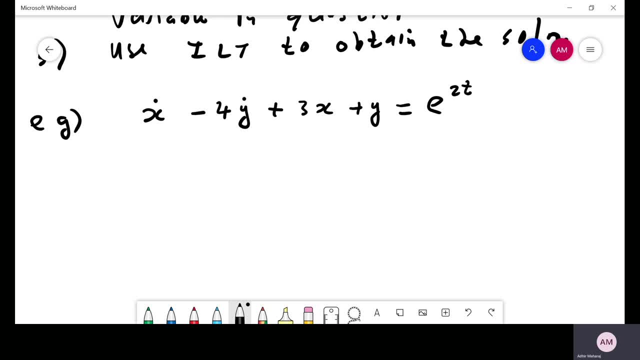 two dependent variables, x and y. so in order to solve for x and y you have to have two equations so we can find nice explicit solutions. so the next equation will be: x dot plus y dot minus x plus 2y is equal to 0 and your initial conditions: 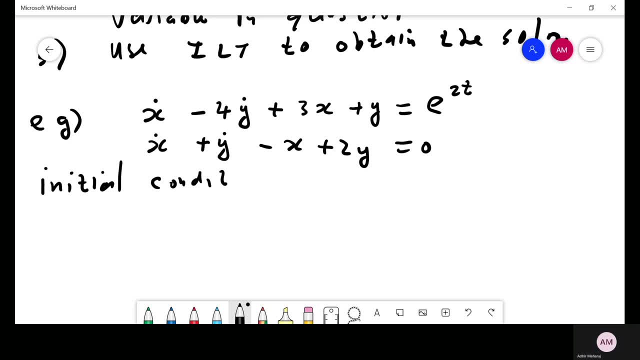 will keep them nice and easy. conditions are: x of 0 is equal to y of 0, which is just equal to 0, right, so we're going to solve the system of equations using laplace transforms. so we will solve. for now, there's two variables here: independent, sorry two. 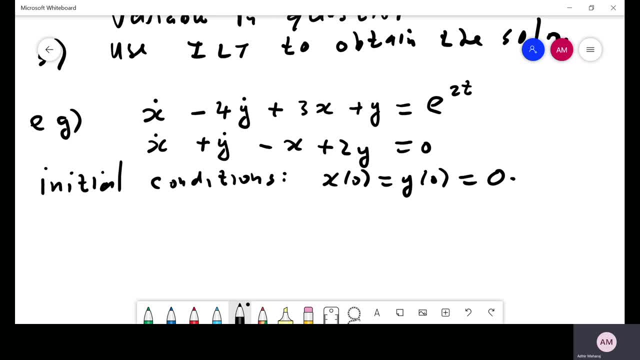 dependent variables x and y. i am going to solve completely for the variable x of t, right, solve for x of t only. however, let's have a look at a different number. so we have a implementation equation again, but again you have an example of an extension in the equation. 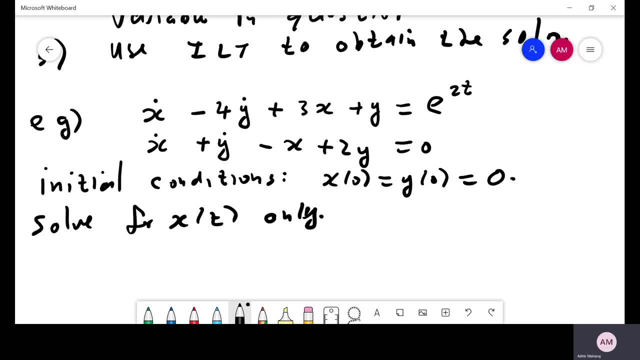 and the answer to the question is self. something let is E, since it doesn't mean everything. well, there is visitors along this table, and so there are many other examples of that. within the equation we have, if an integration equation, there are humans and airt representing both anything other things that require moving things и other things that need to happen in it. for difference in when e and t are trialted. 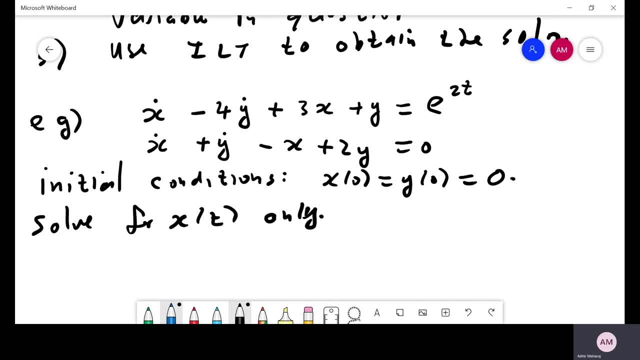 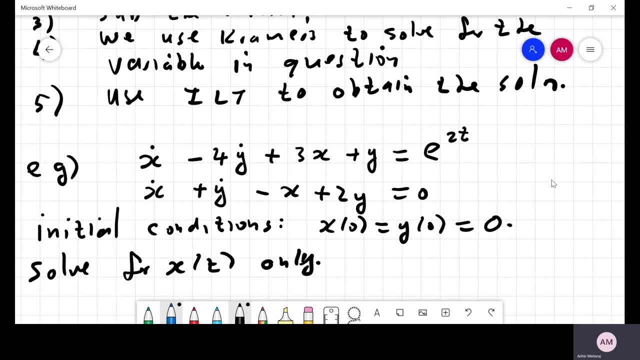 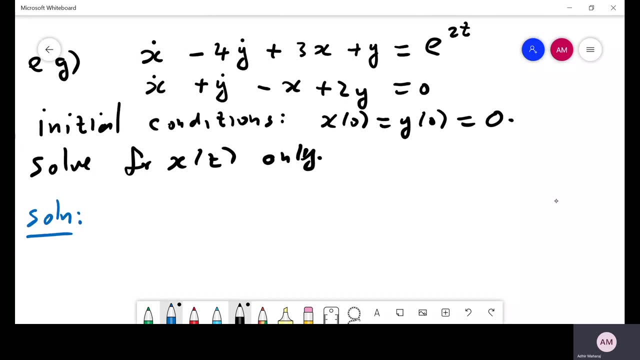 all right. so using laplace transforms and the method i mentioned above, we're going to solve the system for x of t only, right. so the first step is take the laplace transform of the entire system. so let's take the laplace transform of the entire system, so it's going to be l of x dot. 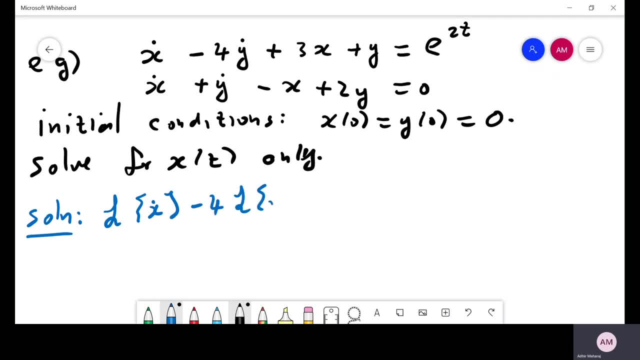 minus 4 l of y, dot plus 3 l of y, plus sorry, 3 l of x plus l of y, and the laplace transform of e to the 2t is 1 over s minus 2. the laplace transform of the second equation will be l. 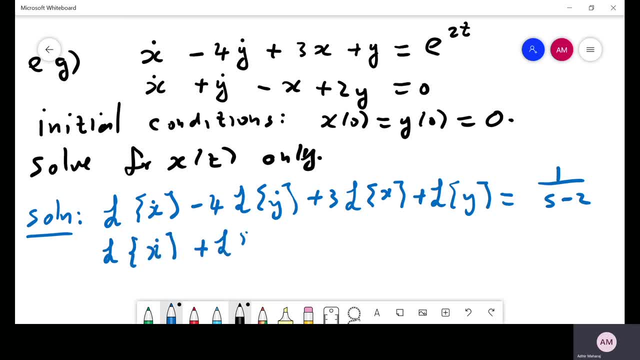 of x, dot plus l of y, dot minus l of x plus 2 l of y, and the laplace transform of zero is just zero, because that's just a constant zero, right? so it's zero over s once you take the laplace transform of the. 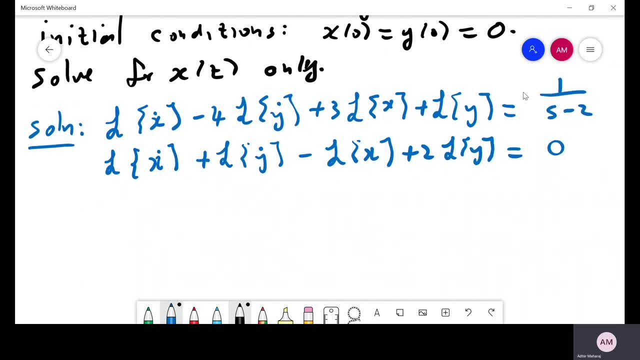 entire equation. the second step of the method is insert your transform of derivatives, that means your laplace transform of derivatives, and in this case, clearly, your highest derivative is the laplace transform of derivatives and in this case, clearly, your highest derivative is x, is dot one, first derivative for y and first derivative for x. so for the laplace transform, the 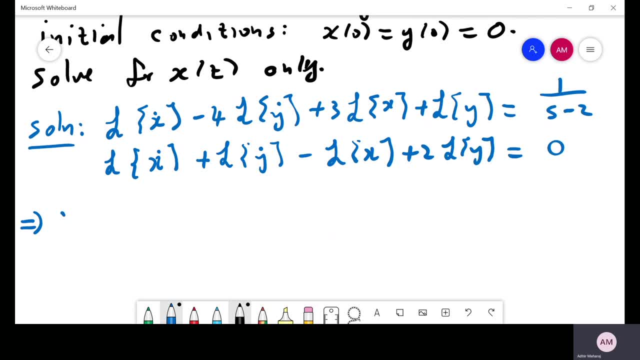 first derivative for l of x dot, it's going to be s. normally we'll say f, capital f of s, but since we're dealing with x, we'll call it capital x of s minus x of 0 minus 4, the laplace transform of y. 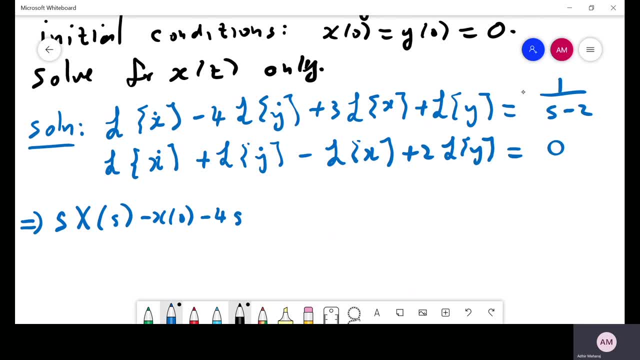 dot will be s capital f of s, but in this case it will be y of s minus y of zero. but don't forget you're multiplying by negative four, so it'll be plus four y of zero. the third term in the first equation is three l of x, which is just three x of s, and the last term on the left hand side. 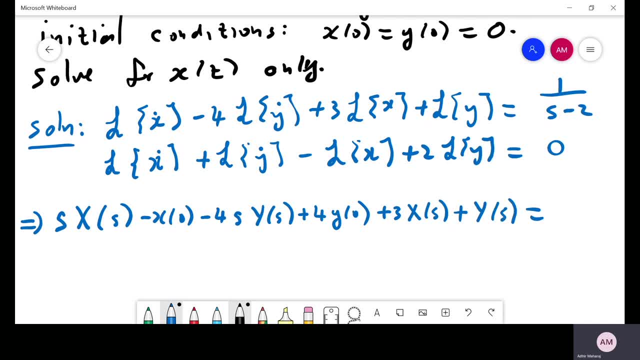 is plus y of s of the first equation, and that's equal to one over s minus two. okay, now we do the exact same thing for the second equation. so l of x dot, so that will be just s capital, x of s minus x of zero. l of y dot will be plus. 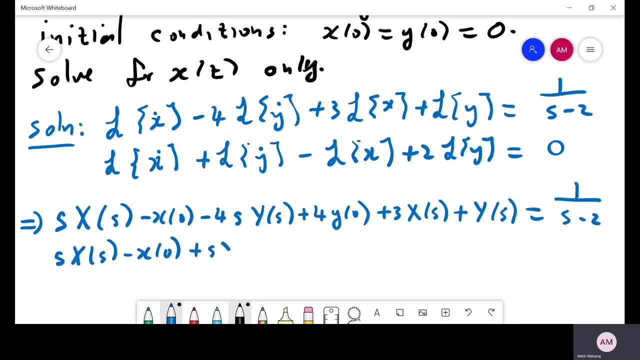 s, l of, let's not say l of y. we'll say y of s minus y of zero, the plus transform of x, the third term, which will be minus x of s, and the last term will be plus 2 y of s, and that's equal to zero. so we have: 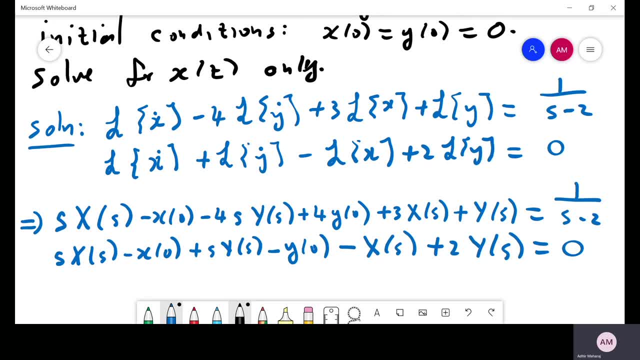 found the laplace transform of both equations. we have inserted a transform of derivatives. so we have completed the first two steps. the third step is to substitute our initial conditions and, if you look at the top of the screen, the initial conditions. we made it a bit easy. x of. 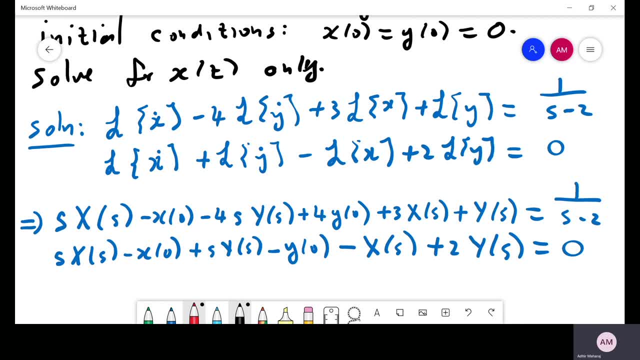 zero is equal to y of zero, which is just zero. so if x of zero is zero, that means that term will just be zero, which means it you can cancel it out. y of zero will also be zero, which means this term is equal to zero. that term is equal to zero in the first equation. in the second equation. 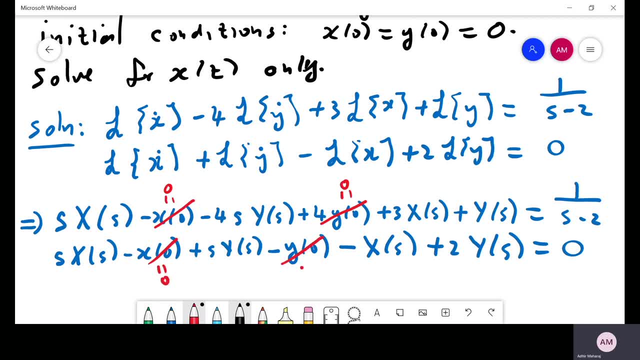 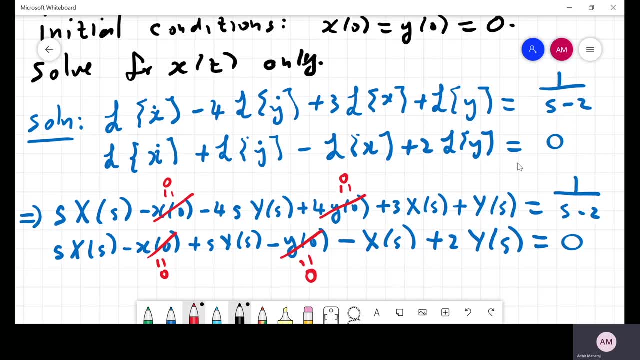 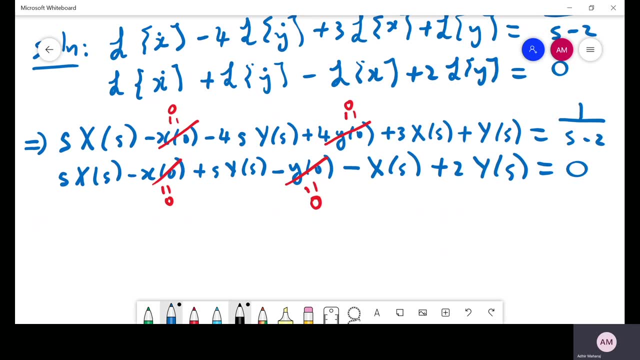 the x of zero is zero, so that's zero. the y of zero is zero, so that's zero. okay, so we have to simplify the equation right, but we didn't simplify completely as yet, because we're going to group the x's together and the y's together and pull out a common factor. 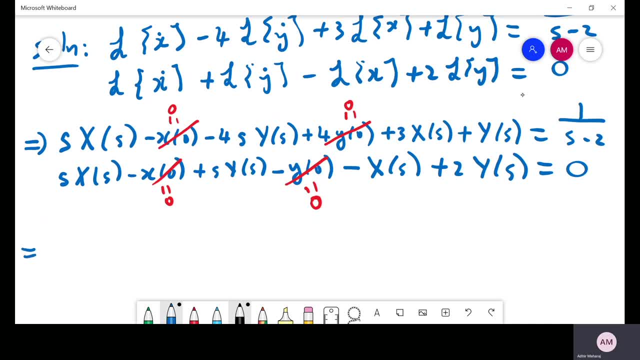 so in the first equation i've got s, x of s and i've got 3 x of s, so i can write that as s plus 3 into x of s. so i pulled out x of s as a common factor for the y's. let's pull out. 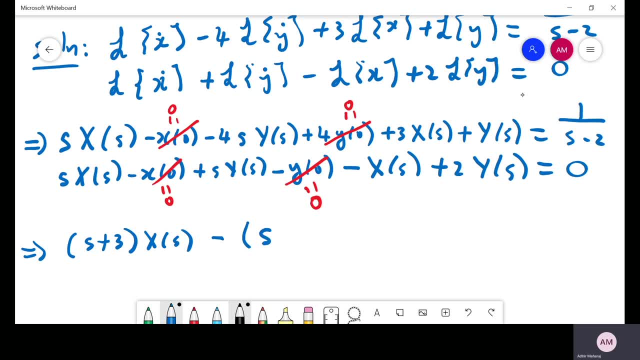 negative y of s, so that will be minus into 4s minus 1. okay, y of s and that is equal to 1 over s minus 2.. so all i did was i grouped the like terms and i pulled out a common factor, doing the same thing for the second equation. so we group the x of s's. 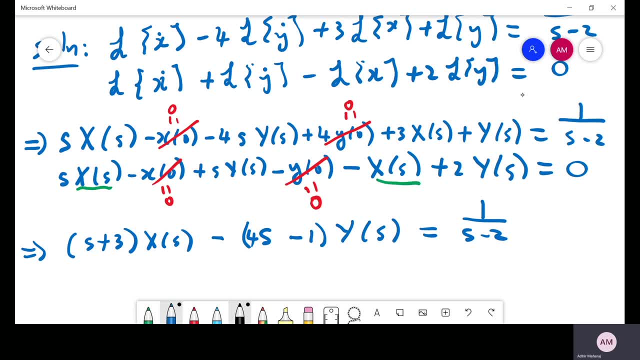 which is this and this, and i pull out x of s as a common factor, so that will give you s minus 1 into x of s. we do the same for the y's that's there and there, so that becomes plus s, plus 2 y of s, and that's equal to. 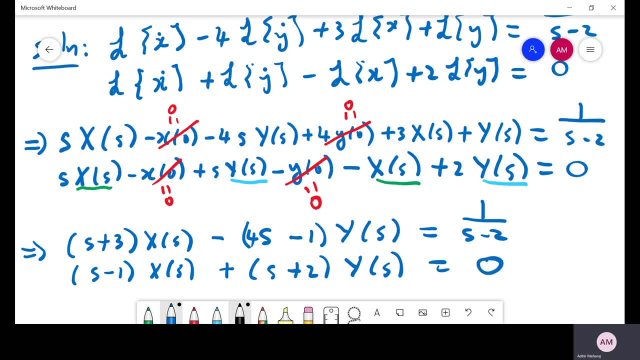 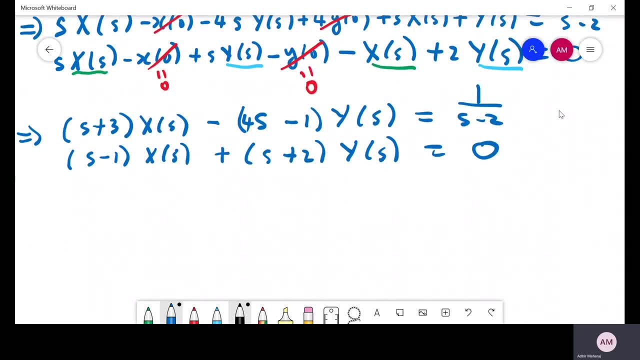 0, right? so now we have a system of equations which is simplified. so remember: system of equations, you can solve it simultaneously or you can solve using kramer's rule. i am going to go with kramer's rule because it's easier, right? so remember, we're solving for x of t, so we're going to use the. 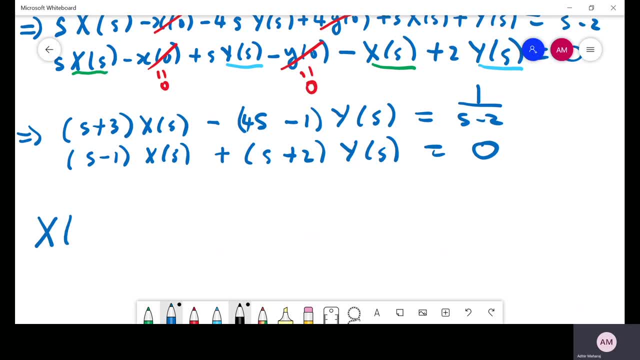 x of s column. so we're going to say x of s is equal to. so according to kramer's rule, you'll replace the x of s column. you notice i always write all the x of s, one below the other, y of s, one below the other. you must do it like that, right. 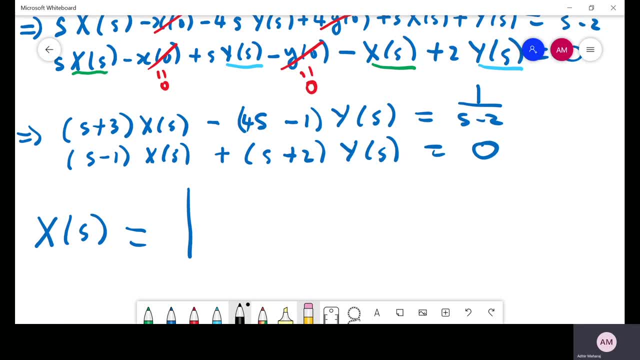 so we can apply kramer's rule easily. so we replace the x of s column with the constants, which is 1 over s minus 2, 0. the y of s column will be minus, into 4s minus 1, which is that all. oh, and you got s plus 2, so that's the determinant of the. 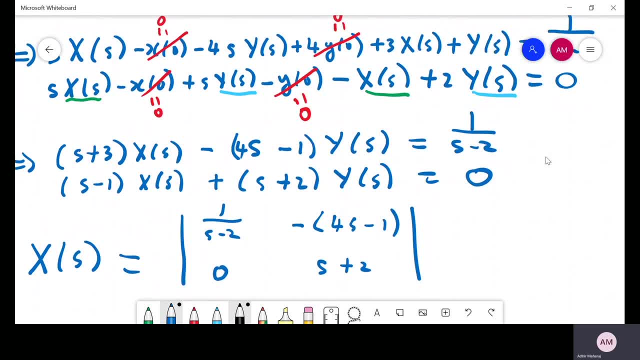 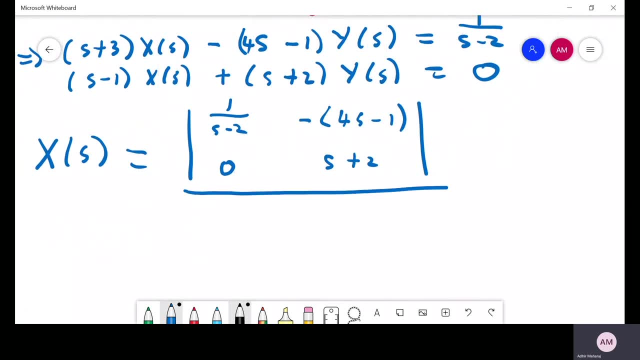 numerator for your when you're applying kramer's rule. okay, next step is we divide that by the coefficient, the determinant of the coefficient matrix, which is s plus 3, s minus 1, minus, into 4s minus 1 and s plus 2.. okay, right, so now we work out the determinant of the numerator and 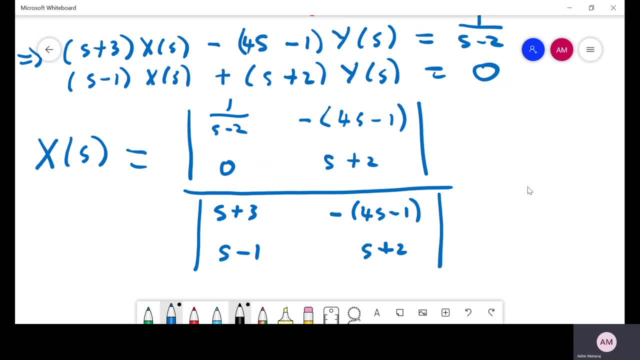 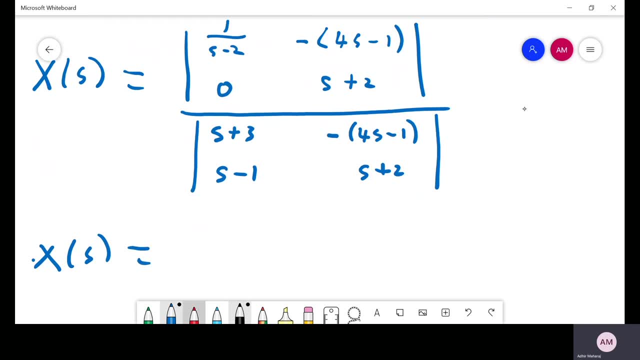 the determinant of your new denominator. so if you have to work that out, that means x of s is equal to. so we cross multiply there, so that gives us s plus 2 over s minus 1 plus 2 over 1, and we cross multiply there. that just gives. 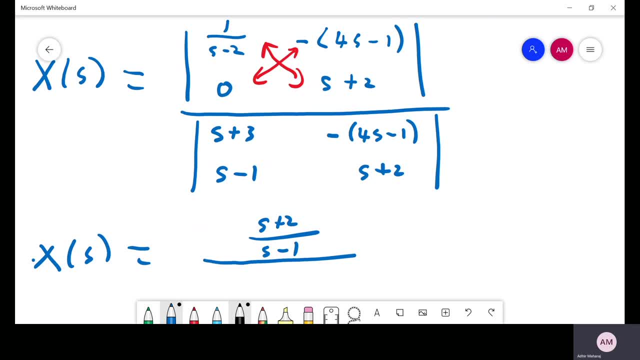 us a 0, all right. so this whole thing will be divided by. so cross multiplying those two terms: right, that will give us s squared plus 5s, plus six, right, and if i and minus the cross product, that would not cross product. cross multiplying negative times negative will make that a positive. 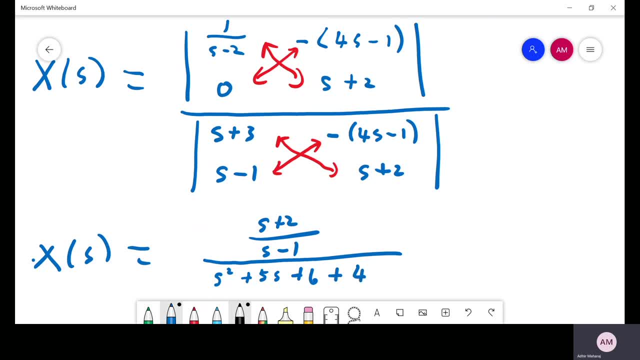 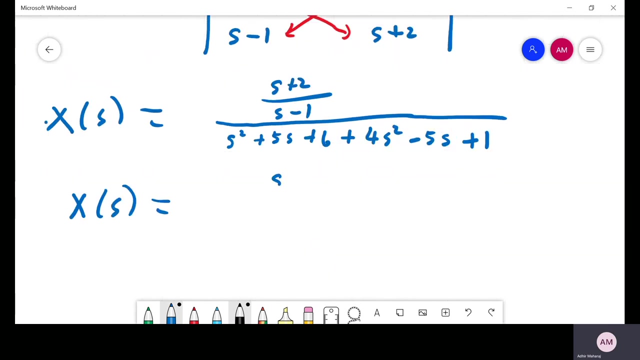 so we'll end up with plus 4s squared. okay, then you'll get minus 4, so that'll be minus 5s, and you'll end up with plus 1, and this can be simplified so we have x of s is equal to s plus 2 all over. i'll take the s minus. 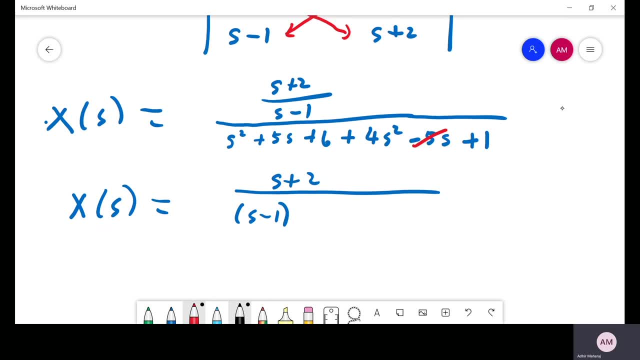 1 to the bottom and we note minus 5s and the plus 5s cancels and you got s squared plus 5s, which is 5s all. for us to find the solution, x of t, we have to take the inverse laplace, transform so x of t will equal to l inverse. 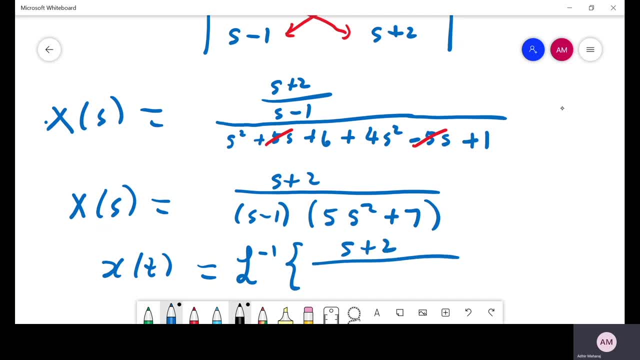 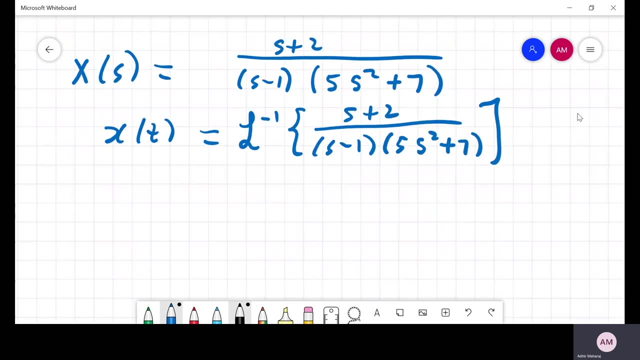 of s plus 2, all over s minus 1, into 5s squared plus 7. okay, so in order for us to find the inverse laplace transform of that, the technique that we're going to use will be partial fractions. so if i we have to use partial fractions here, 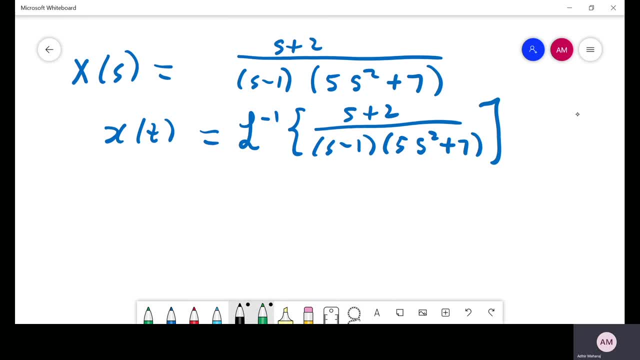 let's say you have s plus 2 over s minus 1 into 5s squared plus 7, so you have a linear factor, s minus 1 in your denominator. so that'll be a over s minus 1. you have 5s squared plus 7. that's an irreducible quadratic factor. 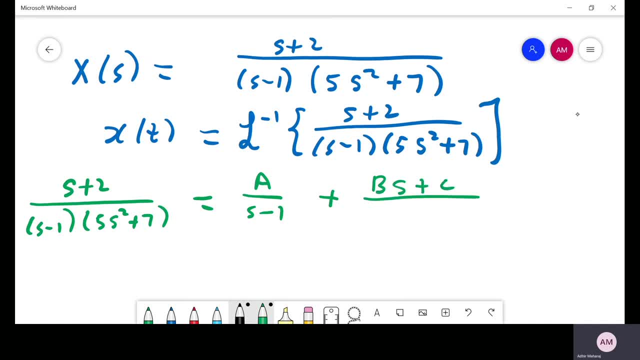 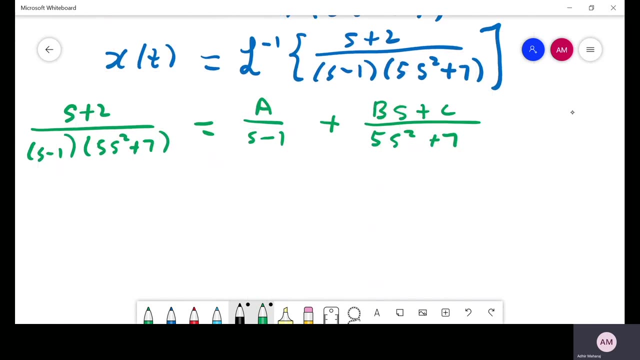 so you'll add bs plus c, all over 5s squared plus 7. we solve for abc in the usual way, like how we did in the previous videos, so that shouldn't take- uh take- you too long to do so. we have s plus 2, getting rid of. 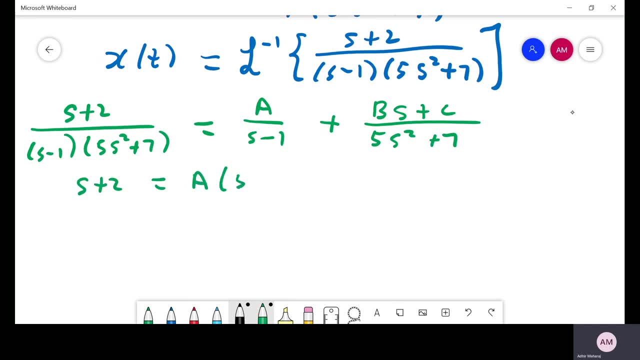 the denominator s plus 2 is equal to a into 5s squared plus 7 plus bs plus c into s minus 1. okay, so to solve, we'll choose s equal to 1. so if i choose s to equal to 1, oops sorry, not s equals. 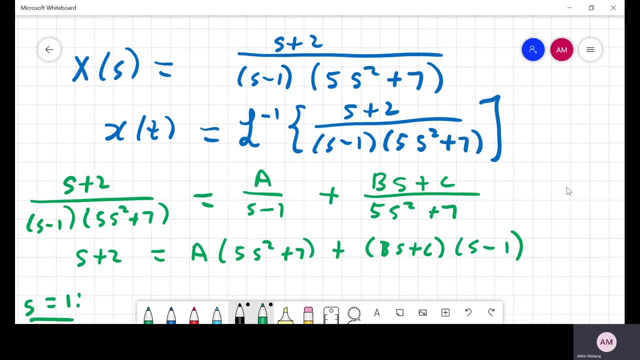 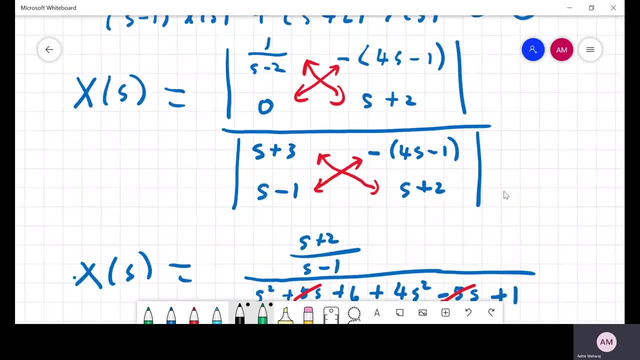 to 1. i think there's a mistake early on. uh, this should have been a s plus s minus 2. okay, this should have been a s. such that, um, if we all write out this, i just can't remember where to go by. right? um, this should have to be the normal viens of r, right? okay, right. 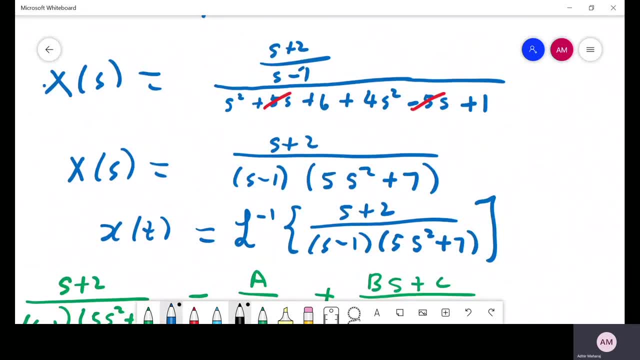 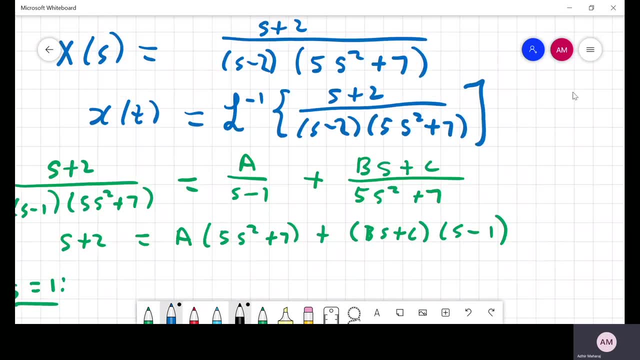 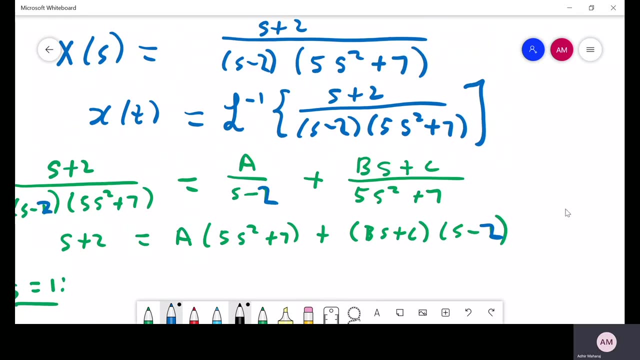 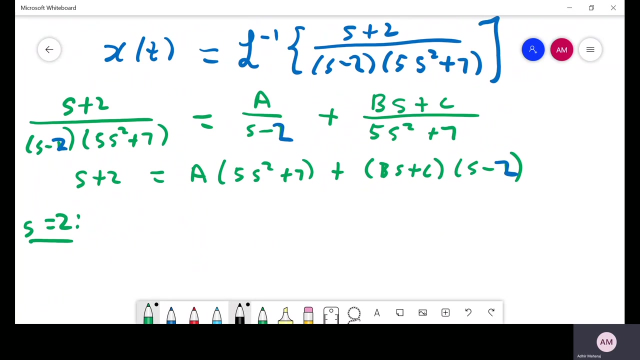 all right. so once again, in this variable, let meto- i'm not going to be stock a- what will be in the other way around- been a s minus two, so let's take the s minus two. there s minus two there, okay. s minus two here, my apologies. s minus two, all right. so then this would just be a two. so if i substitute s equals. 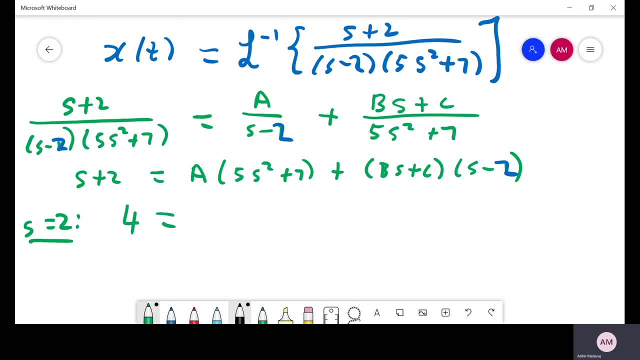 two, you'll get four is equal to substituting four. in the first term. on my right hand side, you'll get 27, a substituting 4. on my second term, on my left right hand side, you'll get 0. so that implies a is equal to 4 over 27.. 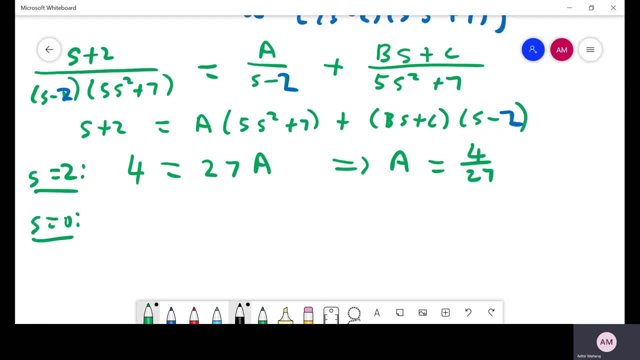 then we can choose: s is equal to 0. if i choose s is equal to 0 on my left hand side, i'll get 2. on my right hand side, if i substitute s equals to 0, i'll get 7a. and if i substitute s equals, i'll get negative 2c. so that implies 2c is equal to a is 4 over 7. so 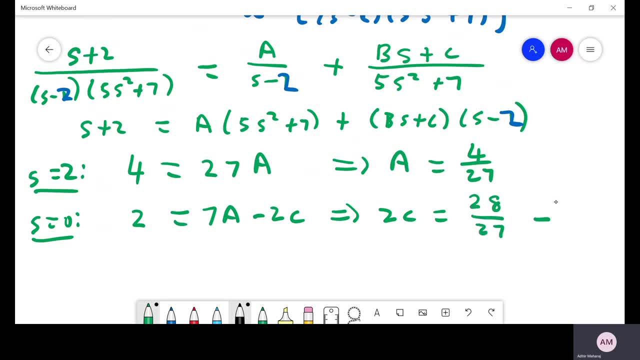 that'll be 28 over 7 minus if i take the 2 to my right right hand side minus 2, which is minus 54 over 27, right, oops? sorry, i don't need to put the minus 54 because i already got the 50 minus sign. so 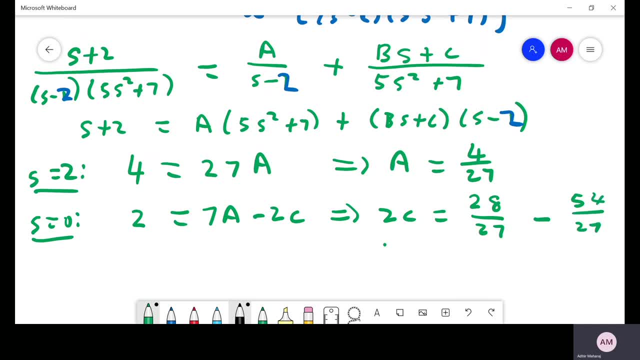 that'll be 54 over 27.. so this means 2c is equal to 26 over 27, which implies c is equal to 13 over 27. so we have a and we have c. okay, so that was pretty easy to do. uh, take, that should be minus. 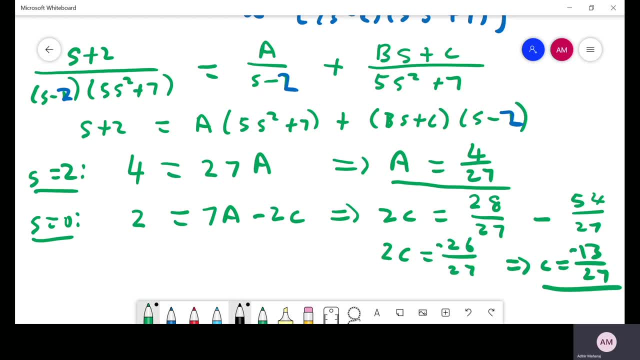 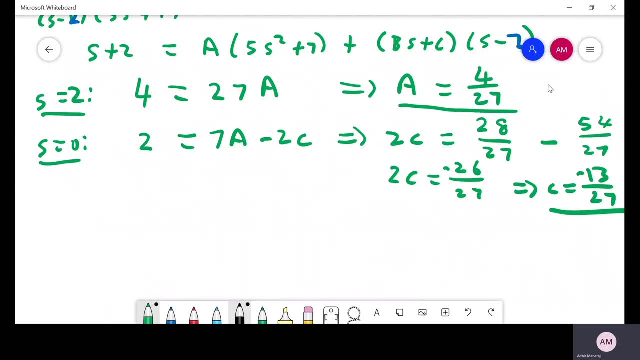 4 over 27. right now we need to just calculate b. so to calculate b, we take the coefficient of. i choose the coefficient of s squared. you'll get 0 on my left because there's no s squared on my right. it's 5a plus b. right, 5a plus b. we know what's a. a is 4 over 27, so it'll be 0 is equal to. 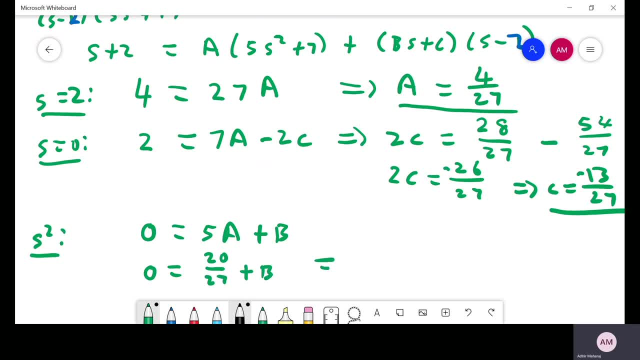 20 over 27 plus b. so that implies b is equal to minus 20 over 27.. okay, so that was pretty easy. we managed to find a, b and c. now we substitute for a, b and c into our partial fractions. so this means, uh, we'll have x of t. 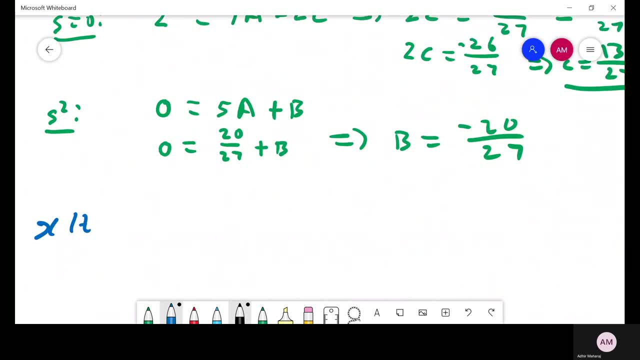 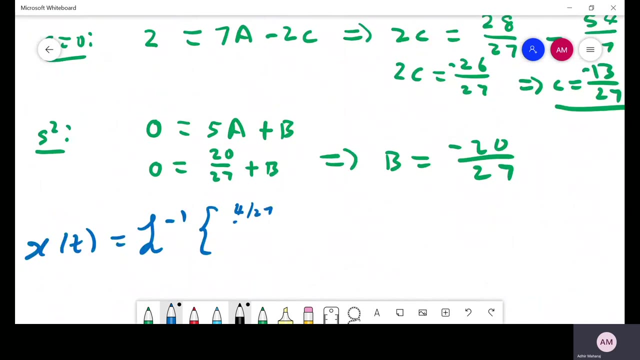 is equal to x of t, that's equal to L inverse a in this case is 4 over 27.. so it will be 4 over 27 over s minus 2.. so it will be 4 over 27 over s minus 2. 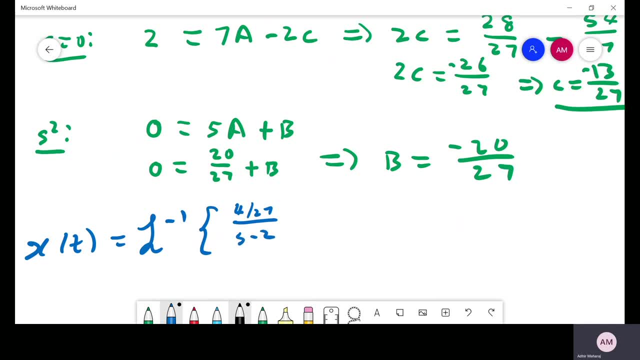 b is minus 20 over 27, so you'll have plus minus 20 over 27s. and c is minus 13 over 27, so it'll be minus 13 over 27 over 5 s squared plus 7. okay, all right, so we now can find the inverse laplace of each of these terms. 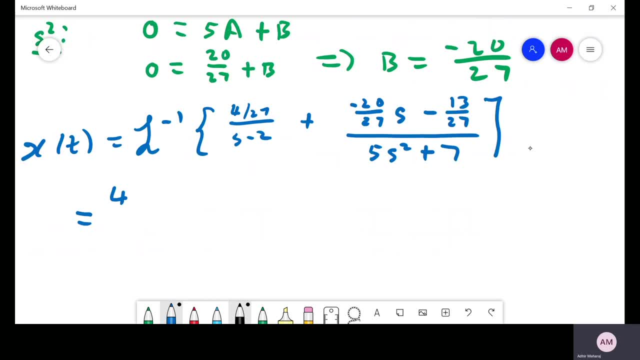 all right, so the first term. if i just split this up, i'll write it as 4 over 27, l inverse of 1 over s minus 2.. that's pretty easy to do. i am going to split the numerator, the numerators in the second fraction, as follows: minus 20 over 27, l inverse of s over 5 s squared. 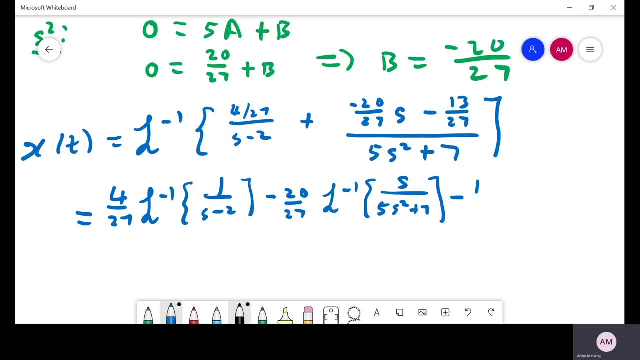 plus 7, and for the next term, i'm going to write as minus 13 over 27, l inverse of 1 over 5 s squared plus 7. okay, now, when you look at this, the first term we can sort out this term here is pretty easy. this is very easy. that sorted out the second term. the problem is this: 5. 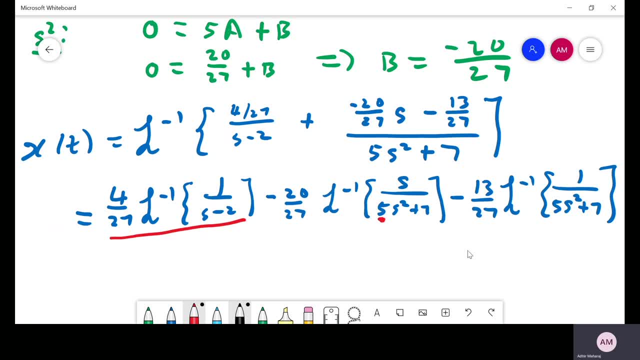 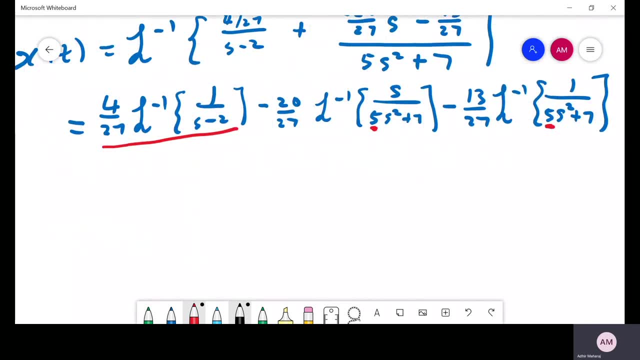 you cannot have 5 in front of the s squared. so what are we going to do? there is, we're going to pull out the 5 as a common factor, and we're going to pull out the 5 as a common factor. we have to do the same for the second term or the third term, right? so this will now become: 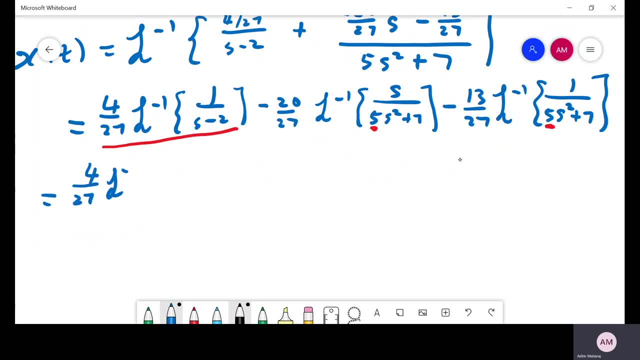 4 over 27. l inverse of 1 over s minus 2. the second term will be minus 20 over 27. so if i pull out 5, technically speaking you from the entire fraction, you're pulling out 1 over 5, so it will become multiplied by 1 over 5. l inverse that will be s. 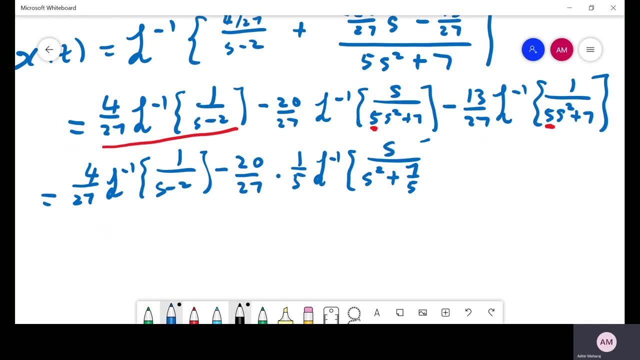 squared plus 7 over 5. all right, the third fraction will be minus 13 over 27. so if you look at the second fraction, now that's sorted out, you can find the inverse of the plus of that very easily. the last fraction will be 1 over 5, l inverse of s squared plus 7 over 5. however, a squared is 7 in over 5. l is 7 over 5. 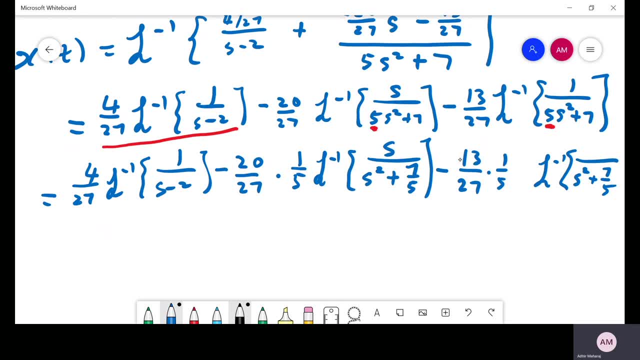 over 5. so my numerator should have a and in this case it will be the square root of 7 over the square root of 5. so if I put in the square root of 7 over the square root of 5, that means on the outside I must put in the square root of. 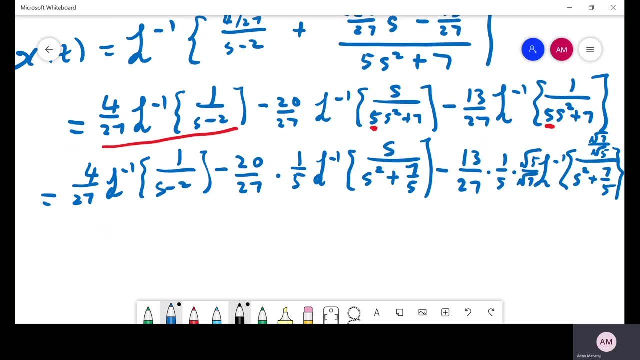 5 over the square root of 7. so the question stays the same. okay, now we can find the inverse Laplace. so this means X of T is equal to the first part, would be 4 over 27. e to the 2t, the second fracture, the second term, will be mind. 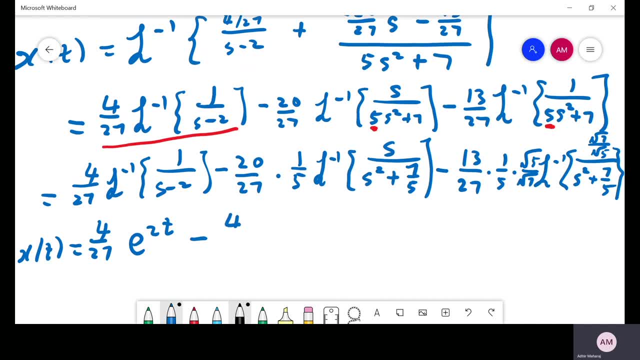 the 20 and the 5 cancels. so that'll be minus 4 over 27. right s over s squared plus seven over four. that's the cost. a is square root of c. seven over five. t. t is under the square root sign. if i have to simplify this, i can write this as: 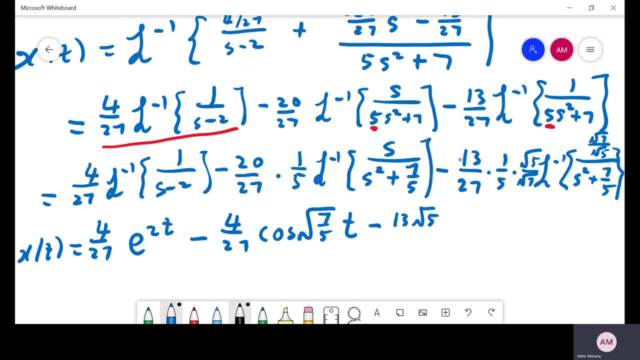 minus 13 root 5 over 5 times 7 is 135 square root 7 and that will just be sine of square root 7 over 5 t. so we now found the solution of uh, the system for x of t. only we only saw now if 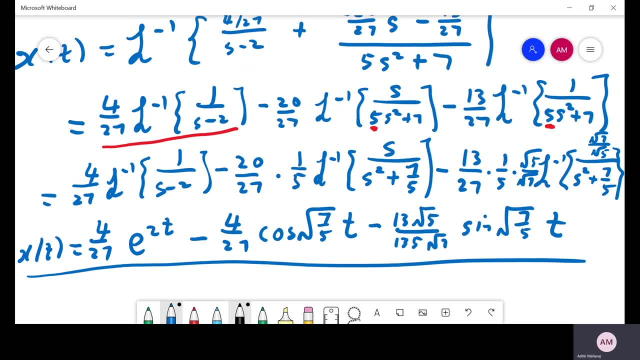 we have to solve for y of t, we'll have to do this entire thing again. and remember: if x of t has this solution, it doesn't mean y of t will have the same solution. so you'll have to do that if it's asked. but we won't ask you to solve for both x and y. 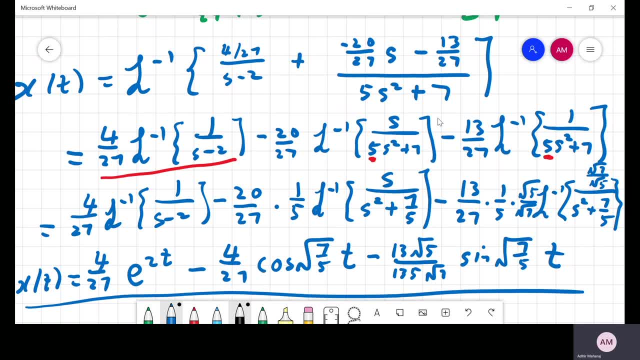 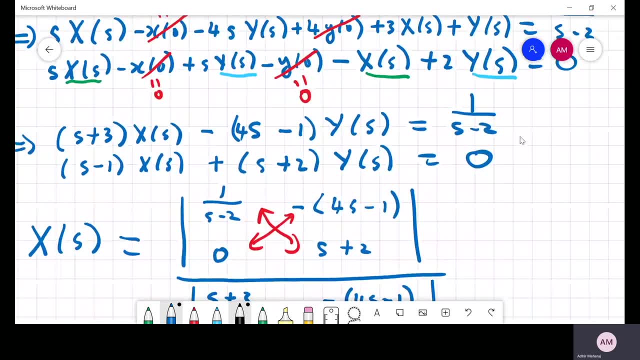 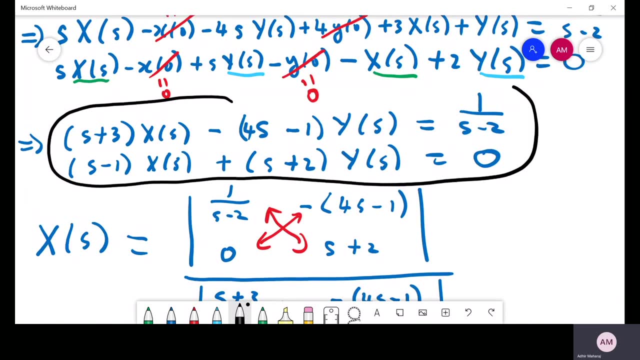 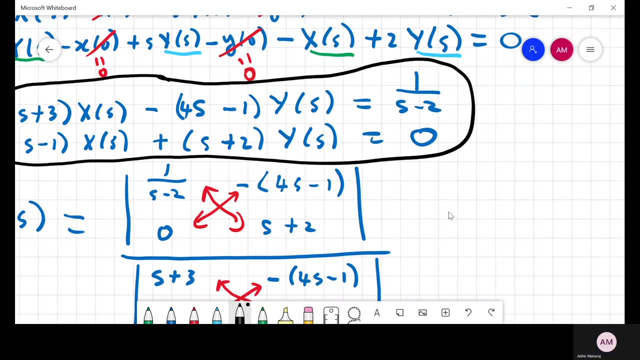 y. but just to give you a heads up, if you have to solve for x and y, like just to practice, the calculation part is already done. till here, right. until here, right. so all we have to do is in the system. if we solving for y of t, let's just move this across, right? if we solving for just y of t, 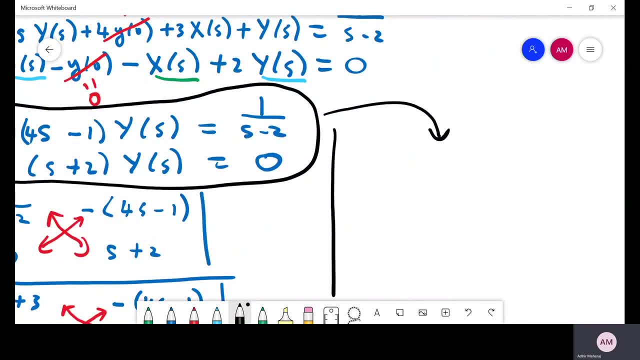 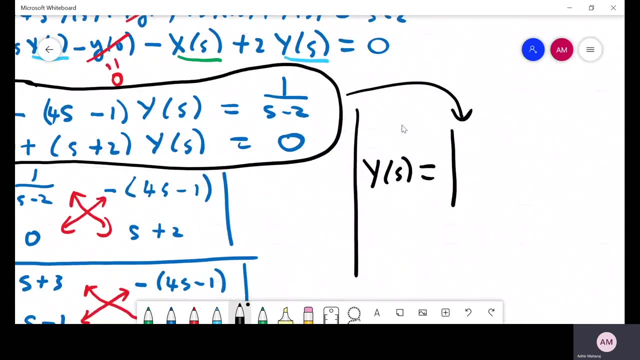 right you'll have, let's just draw a vertical line. you'll say: y of s is equal to the determinant in your numerator. your x of s column will stay the same, so it'll be s plus three, s minus one, s plus three, s minus one. you'll replace the y of s column with your constant, so that'll be s minus two over.